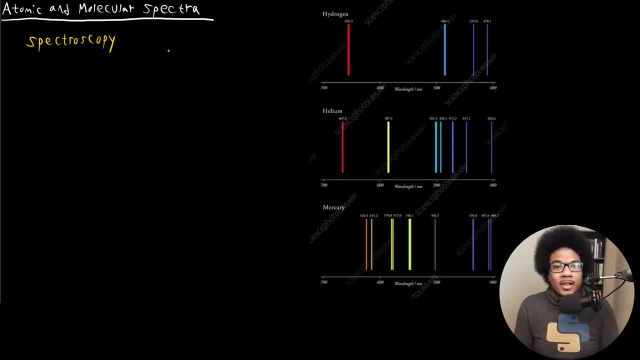 you're looking at the spectrum that's produced when light interacts with matter, right? So let's, for example, let's look at the emission spectra for a few atoms, right? So, basically, what you're looking at is the spectrum that's produced when you shine light on particular. 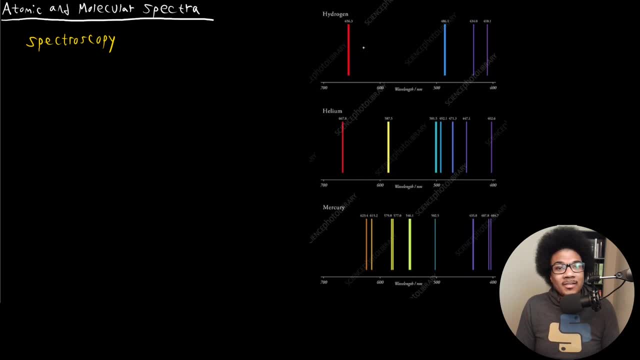 atomic gas samples And this is the. these are the colors that are produced from interaction with that atomic sample And you can see that you don't get a consideration of the spectrum that's produced when you shine light on particular atomic gas samples. And you can see that you don't get a consideration of the spectrum that's produced when you shine light on particular atomic gas samples. 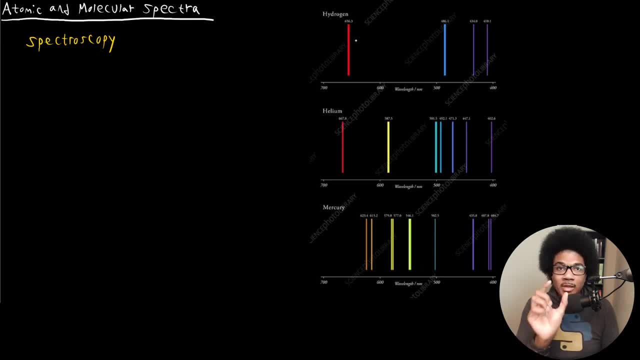 And you can see that you don't get a consideration of the spectrum that's produced. when you shine light on particular atomic gas samples, distribution of light, you get discrete bands at very specific wavelengths right. So the x-axis here is wavelength and it's different for every atom. 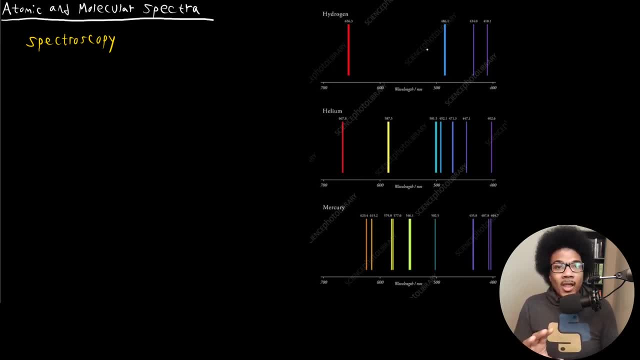 right. So what this gives us is a way to use the spectrum of an atom to identify it. It gives each atom its own spectral footprint, right? So if you see this spectrum, you know that that's hydrogen. it's related to its electronic structure. this is the spectrum of helium, same for mercury down here. 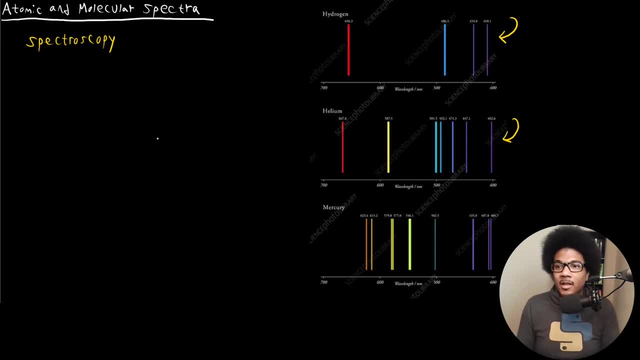 right, they each have a different spectral footprint, um, for what their emission spectrum will look like, right? so how does this tie to the quantization of energy? well, let's think of energy, right, and let's say that you know. so this is like a y-axis: energy increasing, going up, and each of 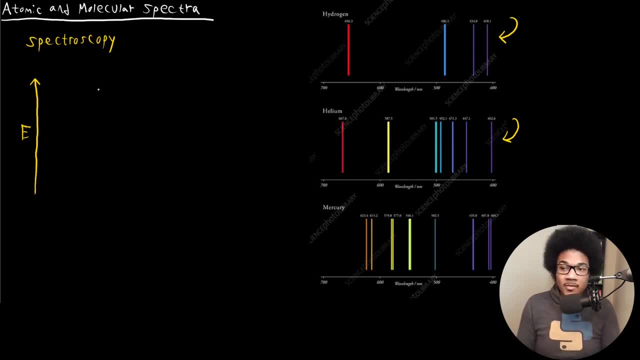 these atoms, any uh species, any quantum system is going to have uh different energy levels, discrete energy levels, right? so i'll label these as such. so we'll have e3 here, we'll have e2 here- i'll make these lines a little bit longer- and e1 down here. 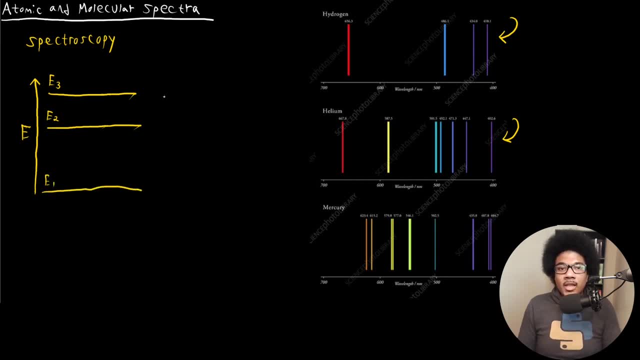 right. so what happens when you excite um, an electron, right? so let's say that there's an electron here, right in e1, and when it's in a higher excited state it's going to relax back down to a lower level, right. and when it relaxes, 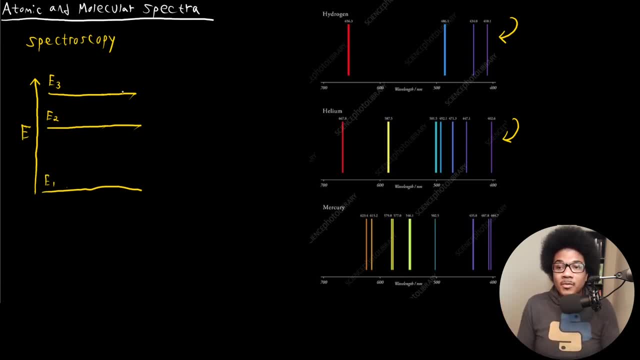 back down. it's what's going to happen is it's going to release a photon right. so if we have an electron relaxing from e3 down to e2, that's going to release a photon right of energy- h nu- and that energy is going to be equal to the gap between those energy levels. so 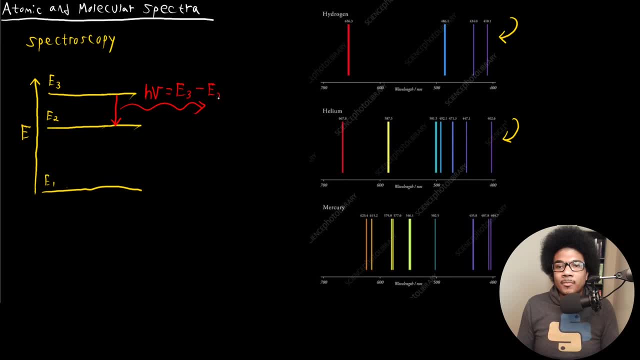 e3 minus e2, right. so by knowing what wavelength of light is, it is um emitted from that, from that atom. you know what's the energy gap between those two energy levels? right, same thing for, let's say, we have um a relaxation from e3 down to e1, right? so if we have a relaxation from e3 down to e1, right. 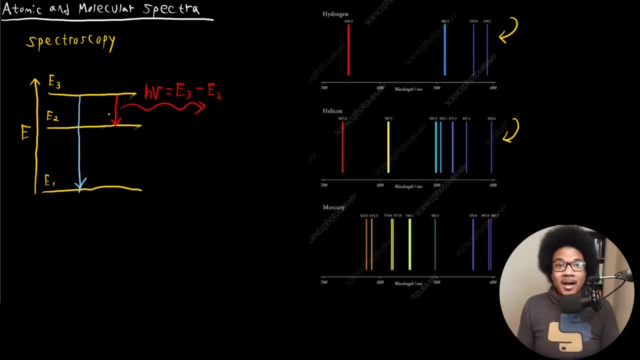 so this is going to be a higher energy um relaxation right, since there's a bigger gap between e3 and e1, so you're going to get a higher energy uh photons. that means going to have a greater frequency, so i'm going to draw this one with a greater frequency. 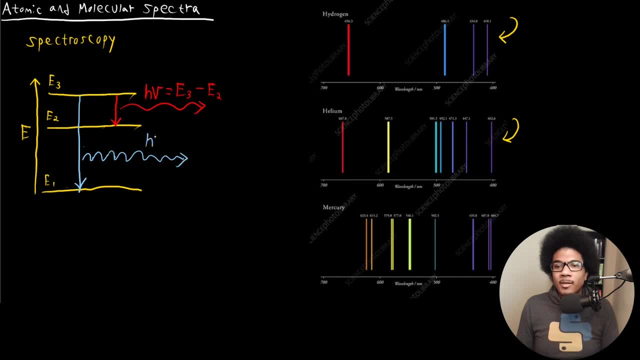 right, but it will still be, you know, h? nu, just with a greater frequency, and it will be equal to e3 minus e1, right? so every single atom have its own electronic structure, right, and using this type of spectroscopy you can figure out what that electronic structure is, right? um, and so this is really the greatest evidence, like i said, that. 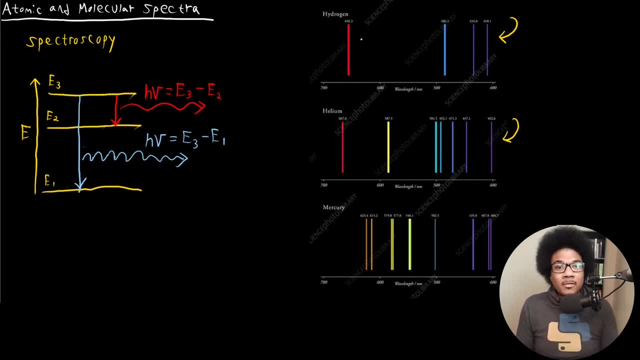 we have of the quantization of energy, because if energy was not quantized, then all of these atoms would produce a continuous spectrum of light, right, uh, maybe they might defer, but it would be continuous. but we see these discrete bands, and so we know that energy has to be quantized. 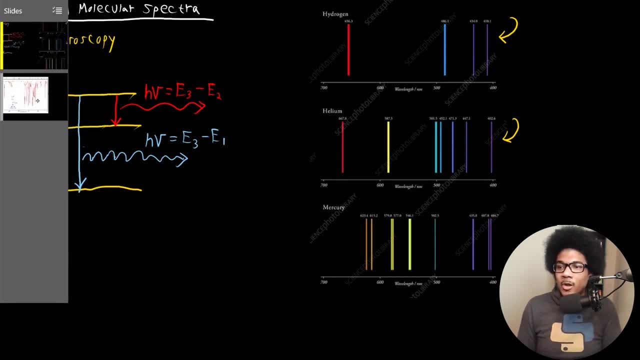 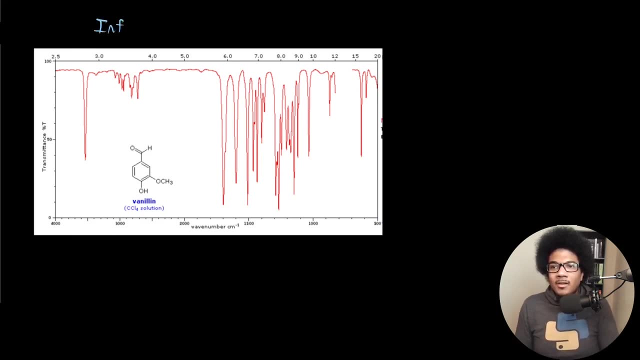 in some way. right now, i want to show you what a molecular spectrum would look like. right? so this is specifically an infrared spectrum, right? so this is shining infrared radiation on a molecule. the molecule we're looking at is vanillin. uh, this is actually the primary extract of vanilla bean. 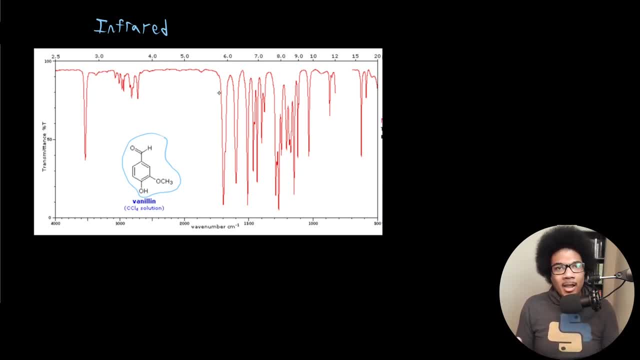 and uh, basically what you're looking at here- i know right now it looks like a bunch of squiggles, but it has the exact same concept, right? if you think back to our video of electromagnetic radiation, when you shine infrared radiation on a sample, you're causing molecular vibrations, right? so 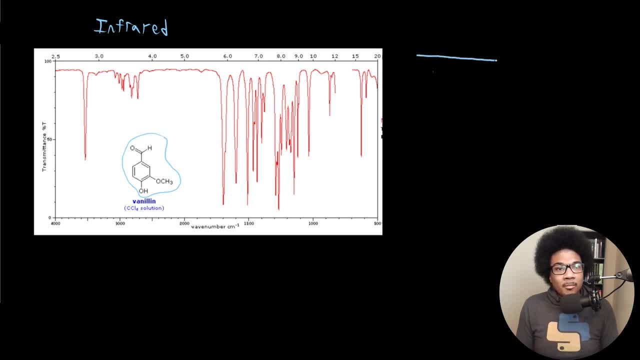 what you're looking at. this is going to be a simplification, but what you're looking at is the uh transition between different vibrational energy levels, right? so let's say, we have some vibrational energy level e2 and e1. right, there's going to be some transition. 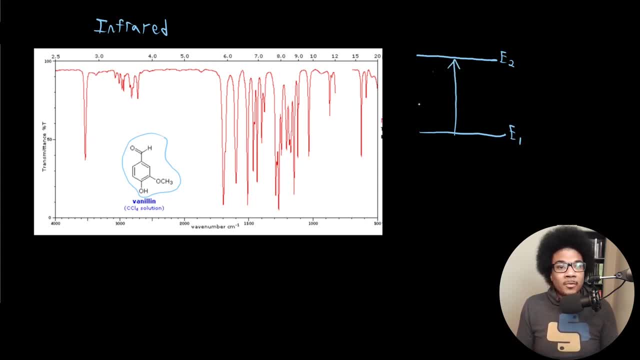 right between e1 and e2. the light that was necessary to excite from e1 to e2 is going to show up as one of these bands on the spectrum right, one of these features in the spectrum right, but you'll notice that it's not continuous right. this um, there's plenty of points of zero. 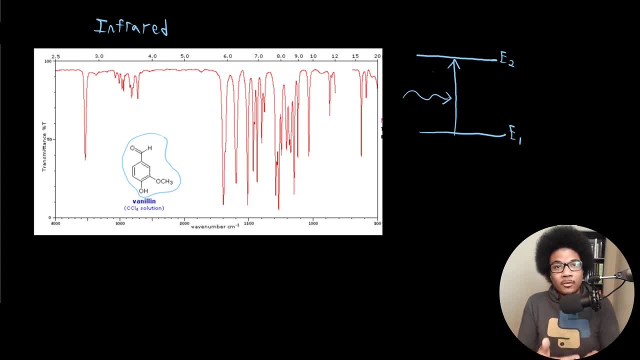 transmittance throughout this spectrum. you're looking at discrete transitions, right? so that's the whole game of spectroscopy. it's trying to look at a spectrum like this and point out a feature like, say: huh, let's see this, this feature here, you know, at uh 3500 wave numbers, right, i'm looking at. 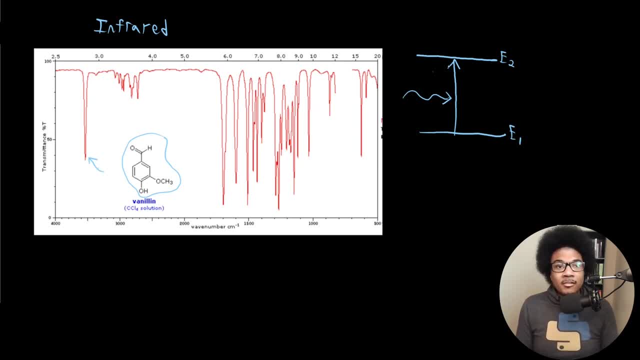 this feature. this looks interesting. can i attribute that to some sort of transition from one vibrational state to another? what? what vibrational state does that have to do with the energy levels that correspond to? and in this case, that would tell you something about the bonding and the structure in the molecule, just like in the atomic spectrum. it would tell you about 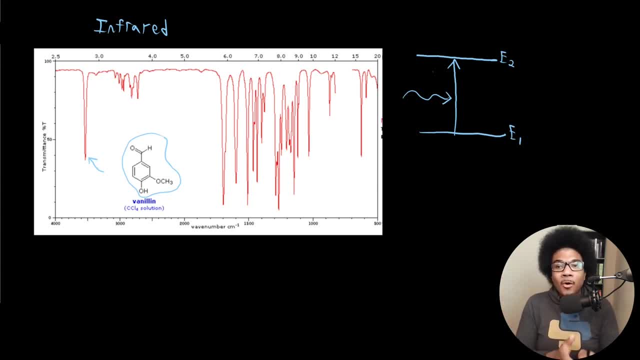 the energy levels of the electrons. right, so that's the whole game of spectroscopy. can i point out some feature and can i relate it to some sort of transition, uh, between discrete energy levels, in this case vibrational energy levels? right, so that's just a quick introduction to atomic and 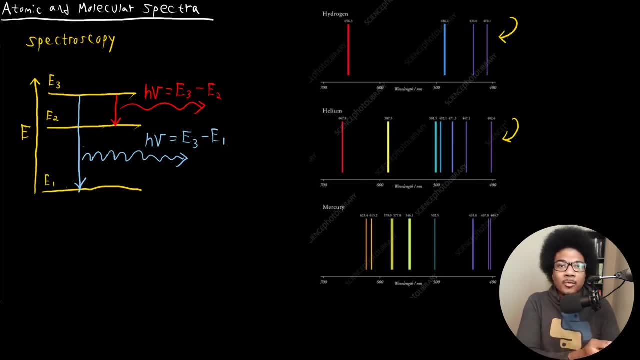 other spectroscopy. we're going to be coming back to spectroscopy throughout this class. when we introduce a new model, it will give us some sort of you know basis for analyzing some type of spectrum so we might like. when we look at the harmonic oscillator model, it is a model of